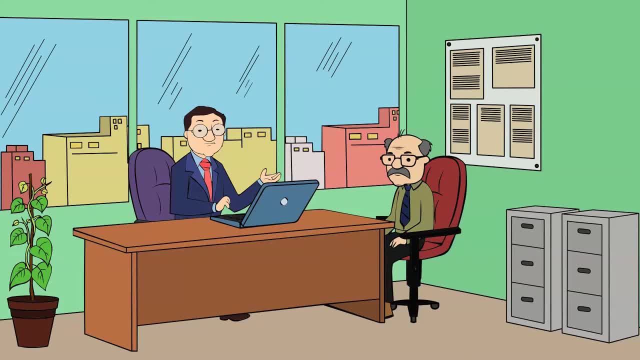 Before committing time, energy and resources to a new project, senior leadership and project managers would want to know: can this project succeed? Is the proposed idea is actually feasible? And even if the project is successful, will the outcomes justify the cost and effort it took to achieve them? Answers to these questions will ultimately decide the fate of the project, And the answers of those basic project queries are determined through a feasibility study. 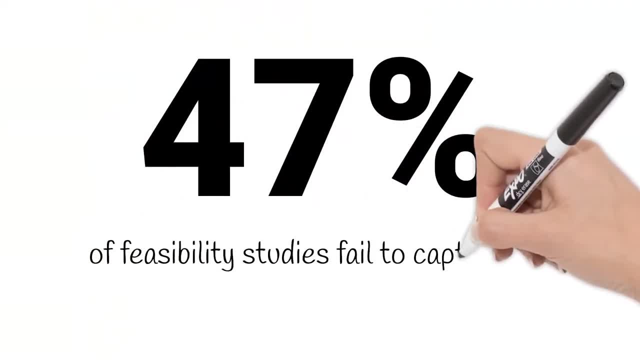 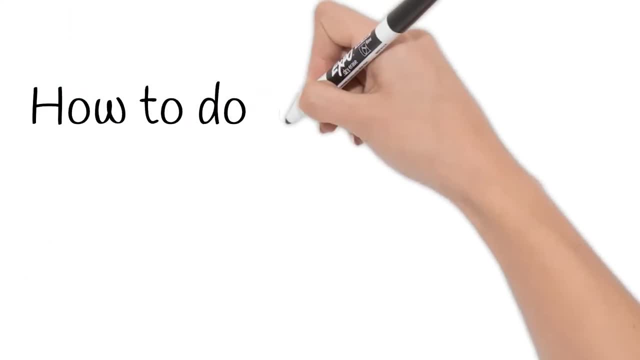 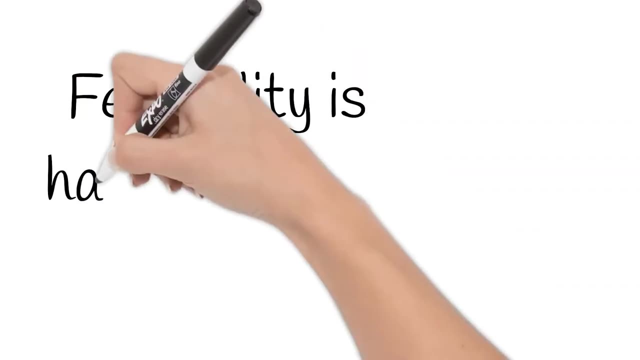 Do you know? 47% of feasibility studies fail to capture key cost aspects of proposed projects. In the next few minutes you will learn how to do a feasibility study for your project in 7 simple steps. Feasibility is hard to prove. The inherent uncertainty makes planning a feasibility study harder than usual. But don't worry, I've got you covered. 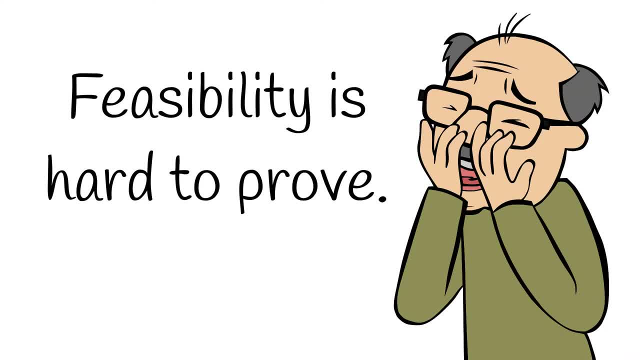 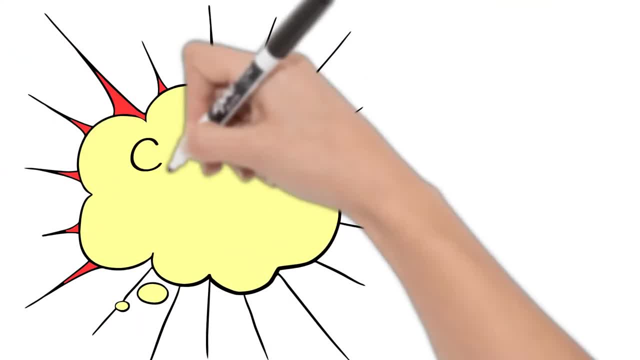 In this video, I would teach you 7 steps technique to conduct effective feasibility. Also, there is one critical factor Which is often downplayed by project managers while conducting a feasibility study. However, this factor decides the fate of your project. 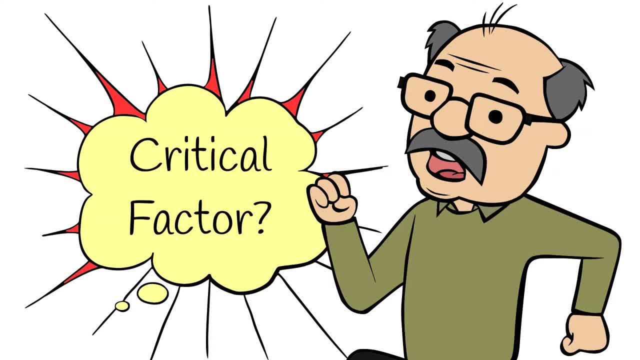 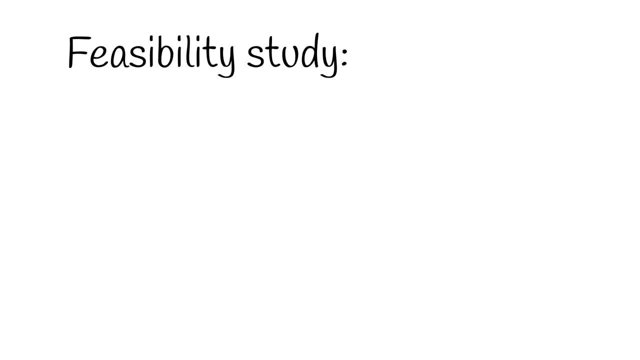 I will discuss this later in this video, So stay tuned. Now, coming to the main question: what is a feasibility study And how to do a feasibility study? Basically, it's an assessment of the practicality of a proposed plan or method. 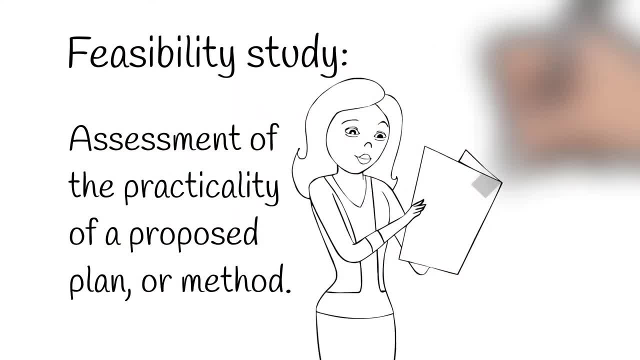 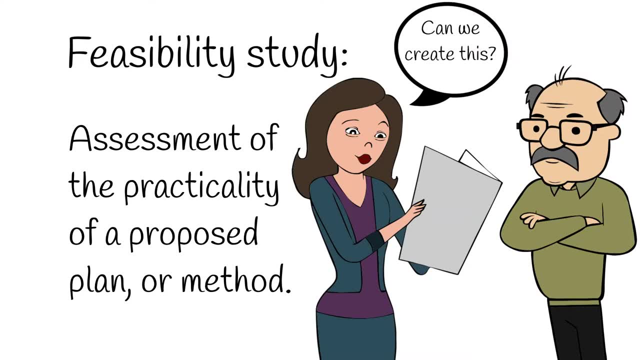 It is. you want to know if this project is feasible- Some of the questions that may generate this, so we can hear people asking: can we create the do this project? The feasibility study helps you and your management team make better informed decisions. 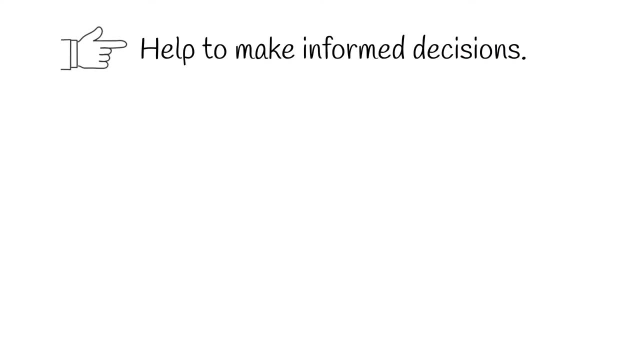 regarding which projects get funded and which get scrapped altogether. A feasibility study analyzes the practicality of a proposed project and assesses how likely the project is to succeed. Typically, feasibility studies are prepared for executives, who will decide whether to green light the project based on the feasibility analysis. 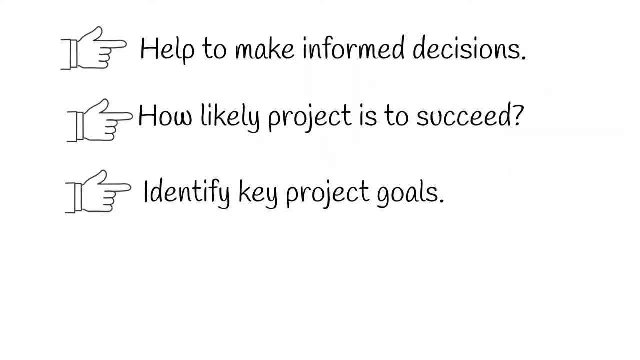 Feasibility studies identify key projects, project goals and relevant factors, examine the market research and detail the resources and budget needed to successfully execute the project. The reason we do a feasibility study is that we need to determine the factors that will make the business opportunity a success. 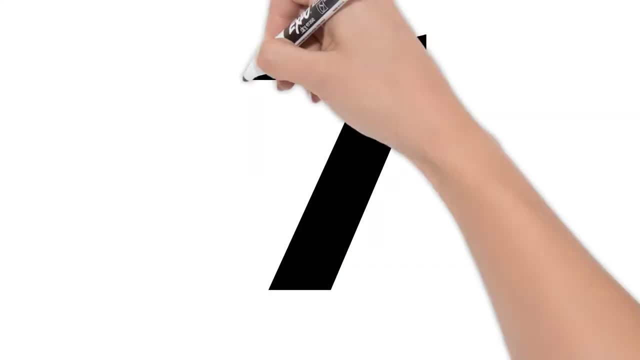 So let's talk about a few steps that we should do in order to conduct the feasibility study. There are mainly seven steps for an effective feasibility study. The first one is preliminary analysis, Just as the feasibility study determines whether a proposed project is feasible. 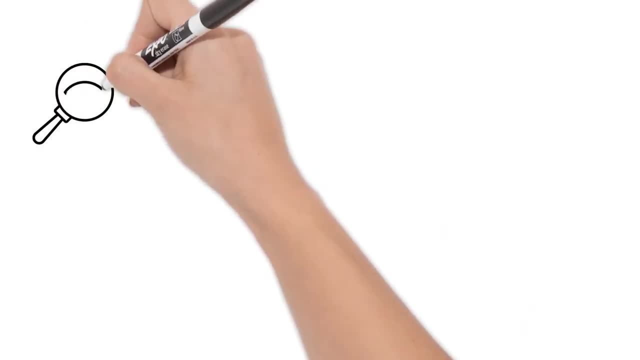 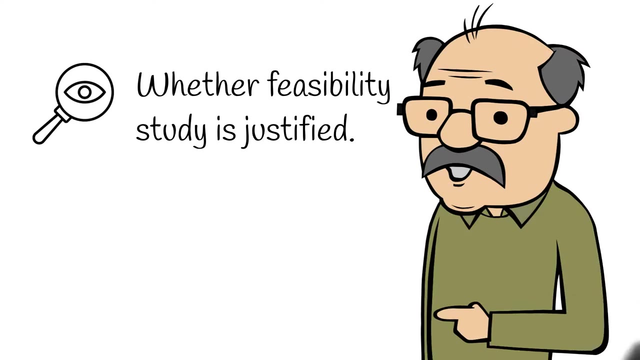 whether a proposed project is worth the effort. the preliminary analysis determines whether the feasibility study itself is justified. The fact is that conducting a feasibility study is an intensive, time-consuming process, and the preliminary analysis will look to uncover any roadblocks that would render the feasibility study useless. 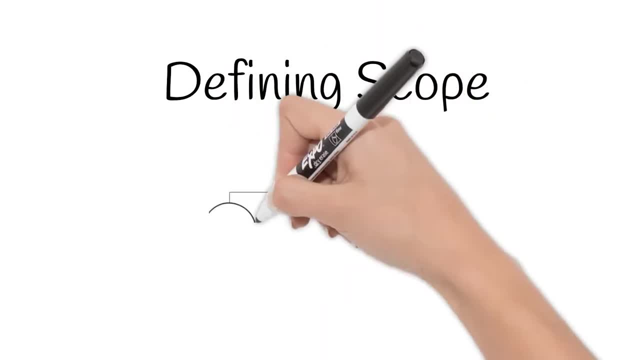 The second one is defining the scope. Before you can determine the potential impact of a project, you have to get clear on the project's scope. This includes defining the project's goals, tasks and objectives, Phases, costs, deliverables and deadlines. 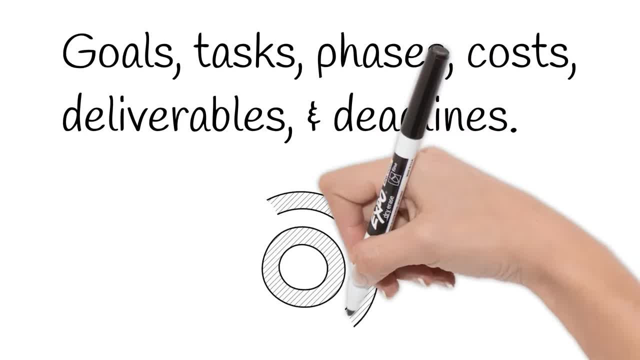 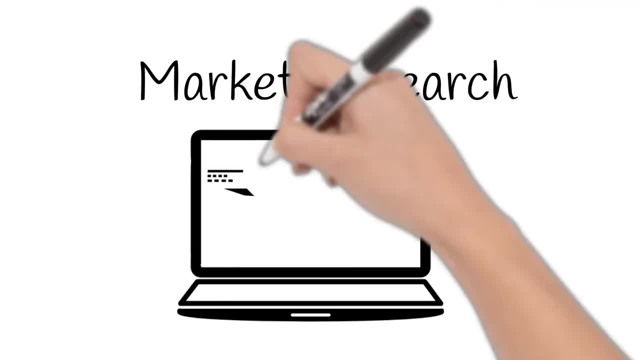 The project scope also identifies internal stakeholders as well as external clients and customers. The third step is to do the market research. Is there a demand for this particular product in the market it seeks to serve? This is critical information to know before committing to a project. 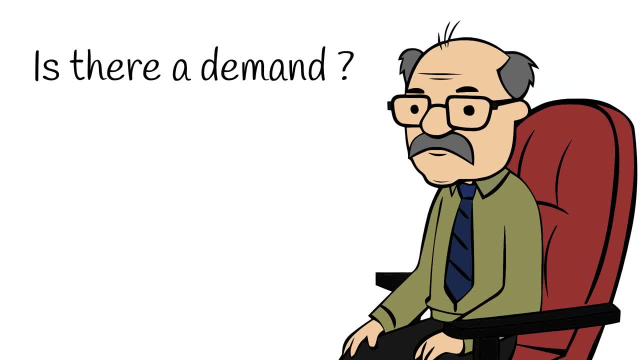 and it's precisely what market research seeks to answer. The market research also gives insight into the current competitive landscape and helps identify factors like geographic influence on the market, the market's overall value and demographics. The fourth step is to perform the financial assessment. 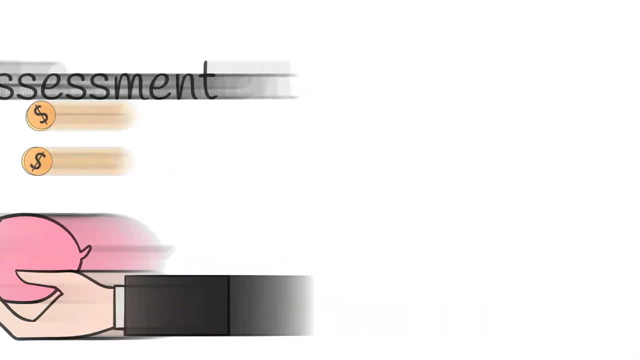 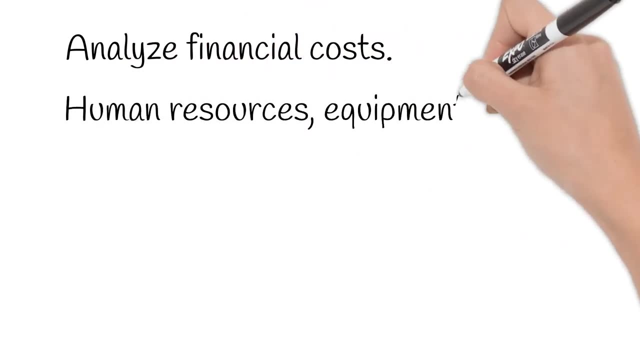 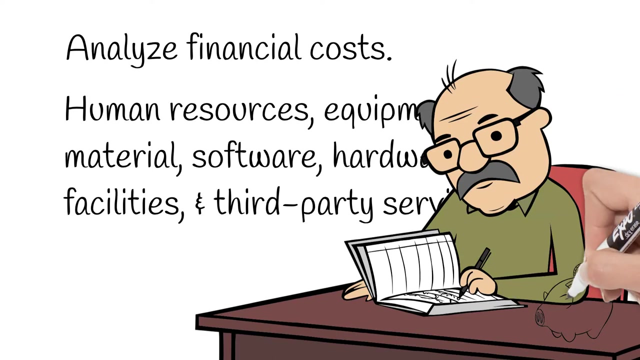 Naturally, the feasibility study will break down and analyze the financial costs and risks involved with the project. Costs may include human resources, equipment, material software, hardware facilities and third-party services. Additionally, the financial assessment will look at the potential impact. 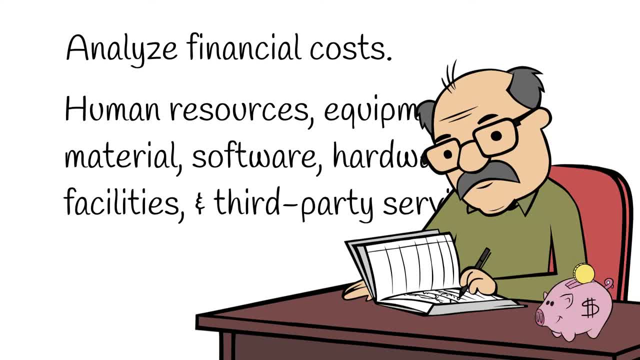 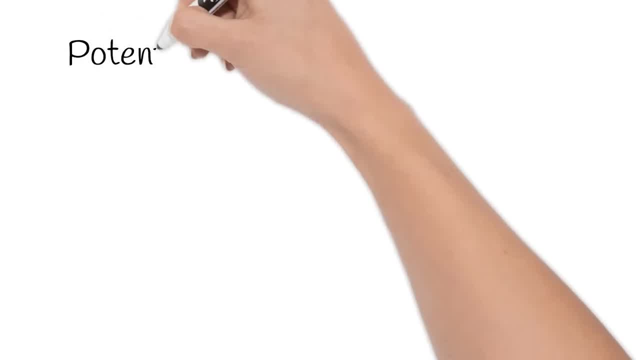 that project failure will have on the bottom line. The fifth step is to perform the financial assessment, Assess risks and alternative solutions. What are the potential problems and circumstances that could lead to project delays or even failure? What are some alternative solutions that would circumvent those problems? 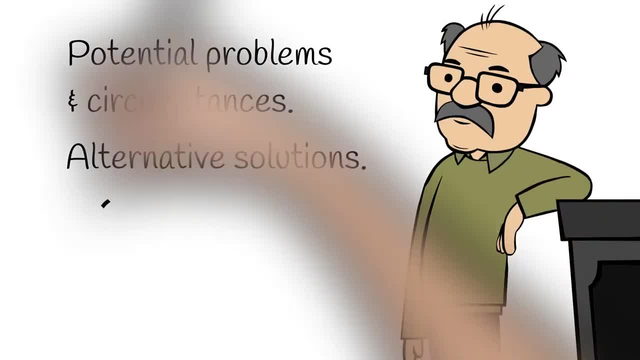 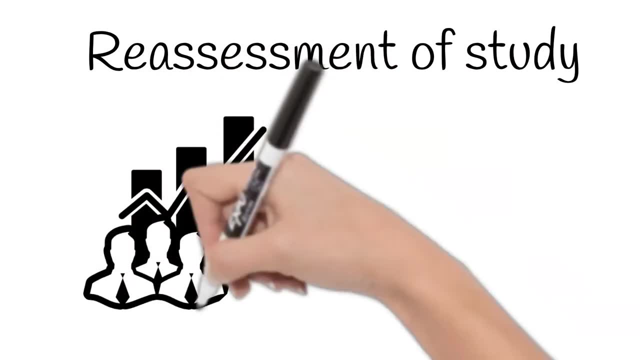 Most feasibility studies will include an assessment of these factors. The next step is a reassessment of a study done so far. At this step, you should seek a reassessment of the entire feasibility study from top to bottom, by a fellow team member, a project manager or other relevant stakeholders. 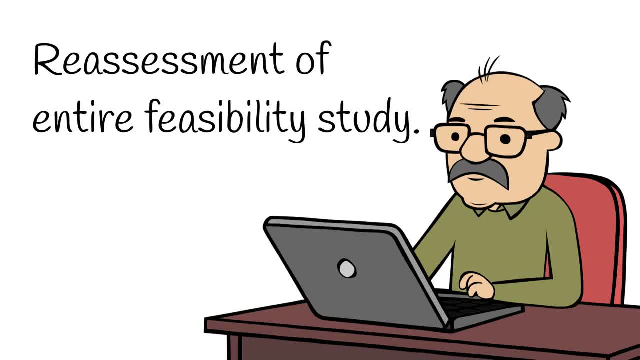 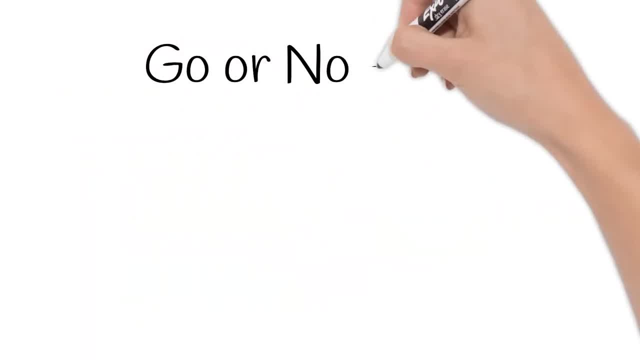 Having a fresh set of eyes on the study will help ensure you don't miss any key elements or miscalculate potential project impacts. The final step is to make go or no-go decision. When it's all said and done, the feasibility study comes down to one decision.